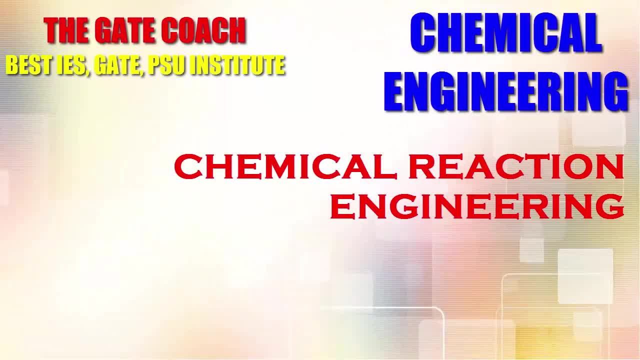 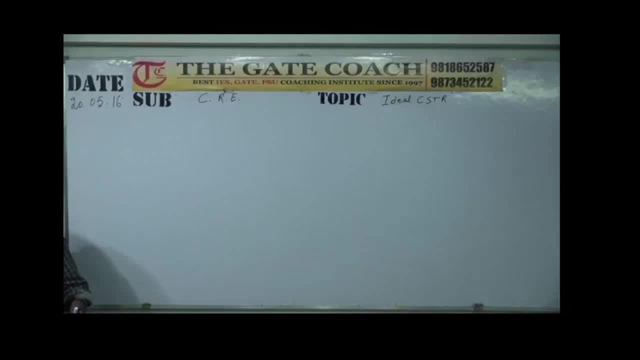 Good morning friends. today we will discuss about designing of ideal CSTR, that is, continuous stirred tank reactor. So first of all I would like to tell you about that construction of CSTR. So it is a continuous stirred tank. reactor means tank, So we have a cylindrical. 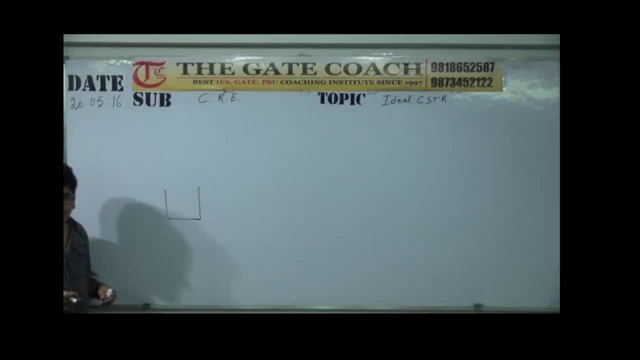 tank like this and continuous stirring is going on. So it simply means there is some agitator or impeller for mixing and continuous stirred tank reactor. Continuous means there is a continuous flow, because CSTR is a flow reactor. Normally we have two types of reactor, as we discussed in last class, One batch reactors. 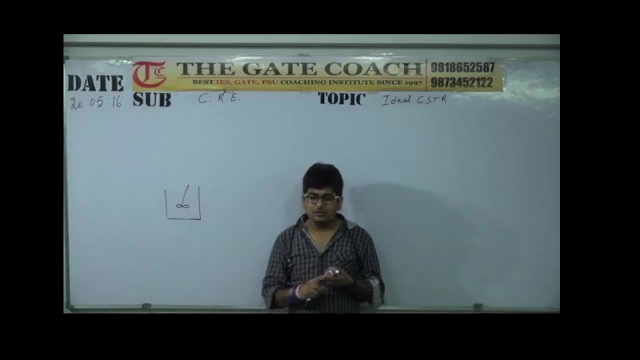 example, is ideal batch reactor and second one is continuous flow reactors. There are two types of reactor we will discuss. First is CSTR and second one is PFR. So today we will talk about CSTR. So in CSTR, since it is a flow reactor, So we have ideal CSTR. 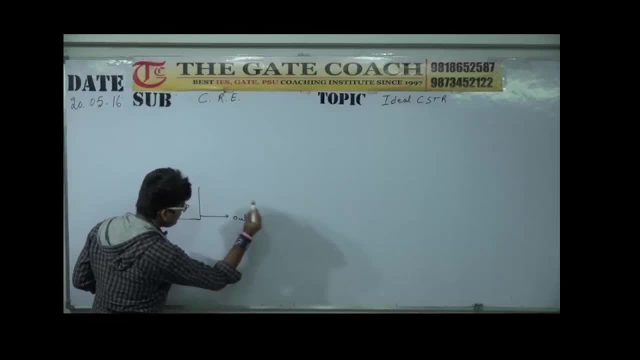 a continuous output stream and you know that output will be continuous only when we have a continuous input to the system. 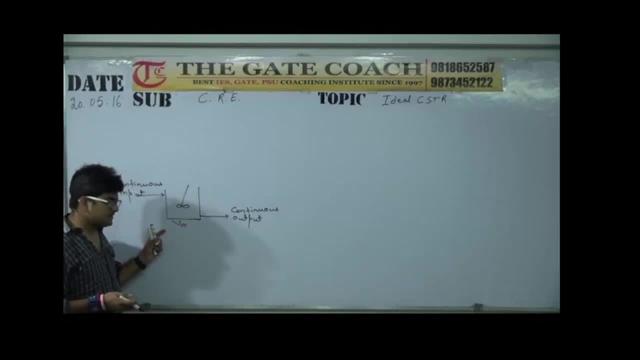 Actually, concentration distribution will be uniform throughout the reactor. reactor concentration distribution will be uniform At any instant of time. the concentration 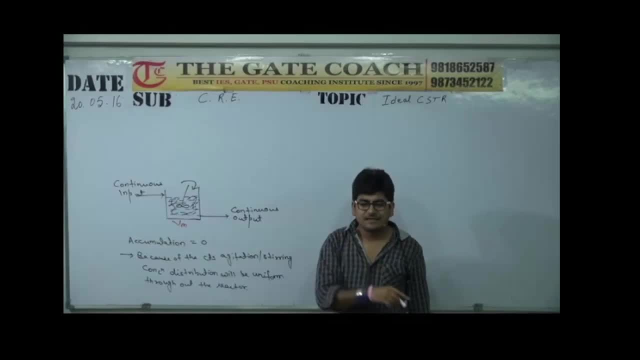 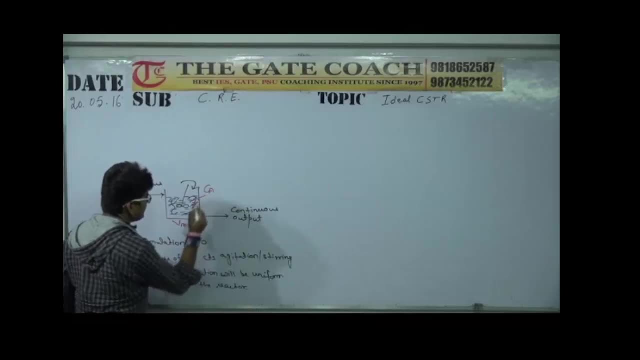 throughout this reactor, at all point of this reactor, will be same. And say that concentration is C means we have a component A and the concentration of component A is C And the initial concentration of that component A was C. A naught The volumetric flow rate of 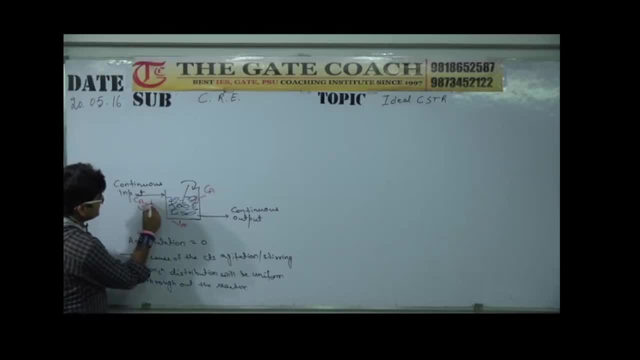 that stream was V- naught and molar flow rate of that stream was F A naught. Because this is steady state condition, the output flow rate will be same as the input flow rate, So volumetric flow rate will be same at exit, which is denoted by small v And obviously. 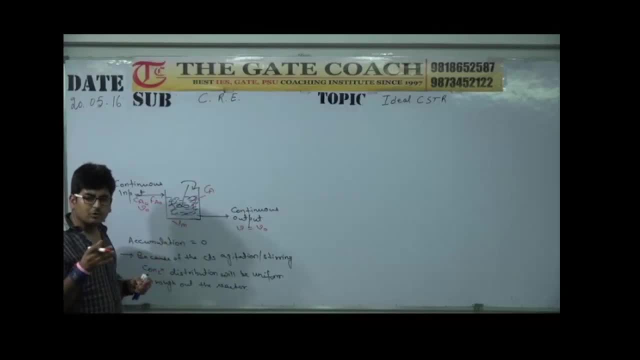 molar flow rate will change because some moles will disappear in the reactor. Some moles will take part, So that is why the molar flow rate will change in this reactor. So this is clear to all of you. So one more thing I like to tell you that we say this is a mixed flow reactor. 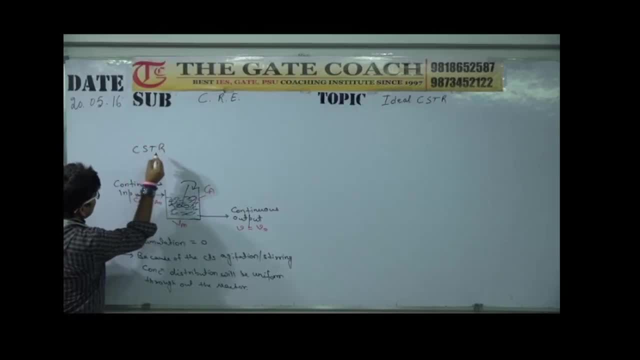 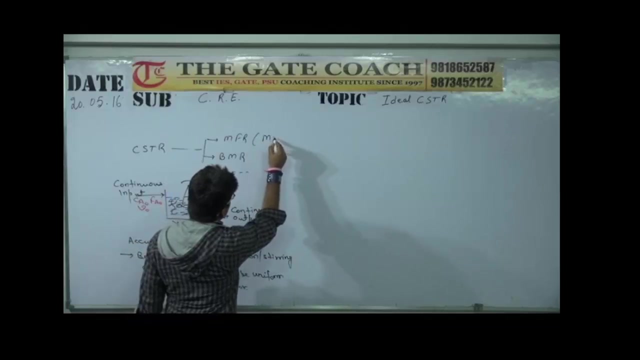 This is a CSTR, And CSTR is also known as MFR, BMR, etcetera. MFR means mixed flow reactor and BMR means back mixed reactor. mixed flow reactor, because it is a continuous flow reactor and there is continuous mixing. 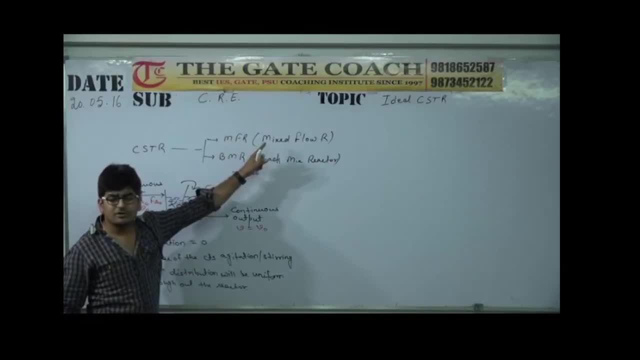 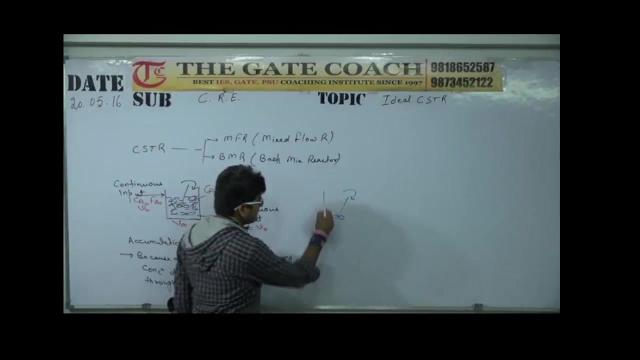 going on in this reactor. That is why it is known as mixed flow reactor and it is also known as back mixed reactor. Why So? in simple words, I would like to tell you that this is an impeller. It rotates like this and this tank, this point is input and this point is 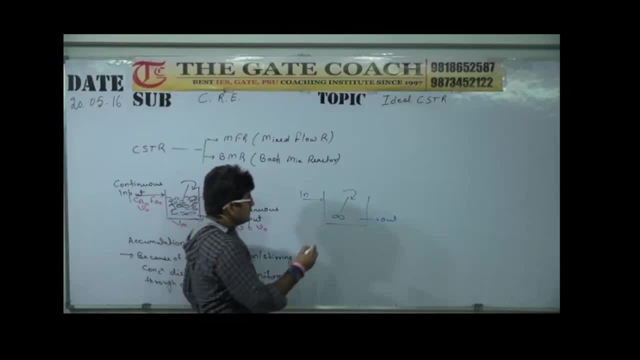 output. So there are some new molecules, suppose because of, from this inlet stream and there are some old molecules in this reactor near to the exit stream, near to the outlet. So because of this rotation of the impeller, some of these molecules flow back towards. 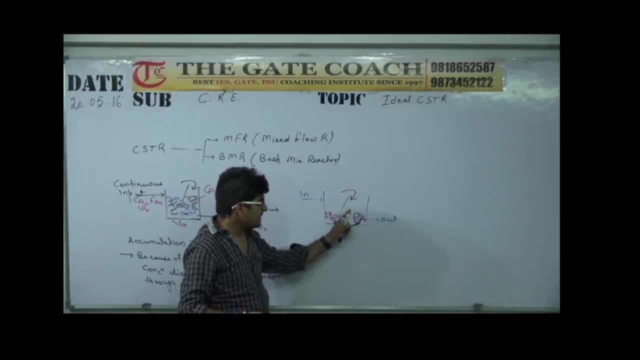 the inlet, and these molecules which are near to the outlet, in this case these molecules interact with these molecules which are just entered in this reactor. So simply, you can see that some of the molecules are coming back from the output side in backward direction. 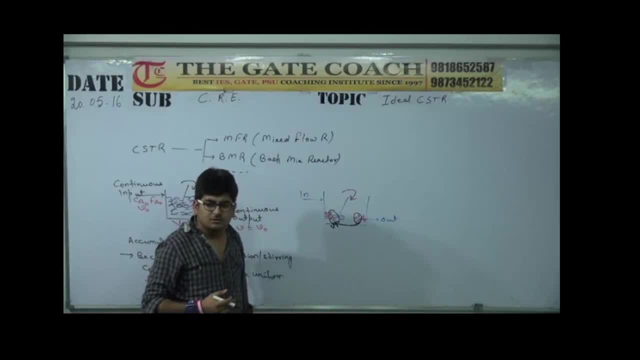 and they are interacting with the inlet molecules. So this interaction of molecules is mixing and because output molecules are coming back to the inlet molecules, so that is called back mixing And this reactor is known as back mixed reactor. So because of this backward mixing, 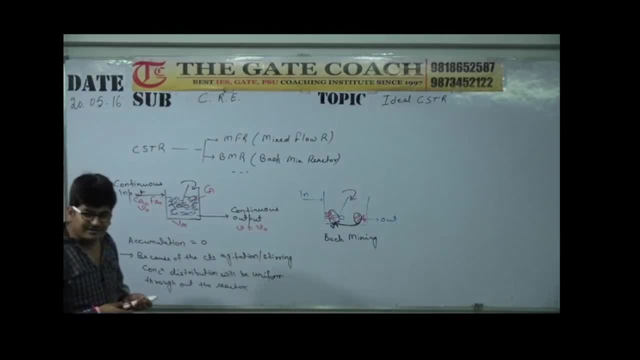 this is called back mixed reactor. So this is something about your ideal CSTR. So there is one point you should know that. remember that because of the continuous agitation, concentration distribution throughout the reactor is uniform. So it means 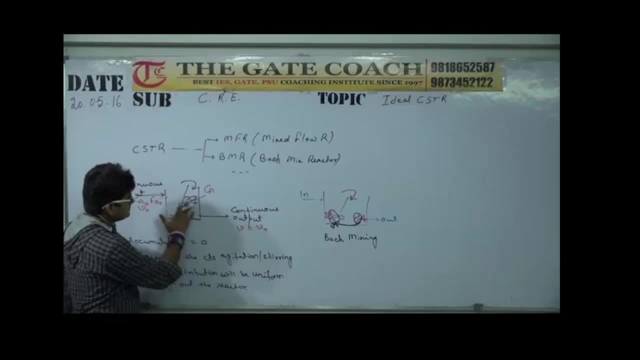 and the concentration in the reactor is C- A, So concentration distribution throughout the reactor is uniform. It means near the outlet valve. also the concentration will be same as that of in this reactor. So it simply means concentration of A at the outlet. 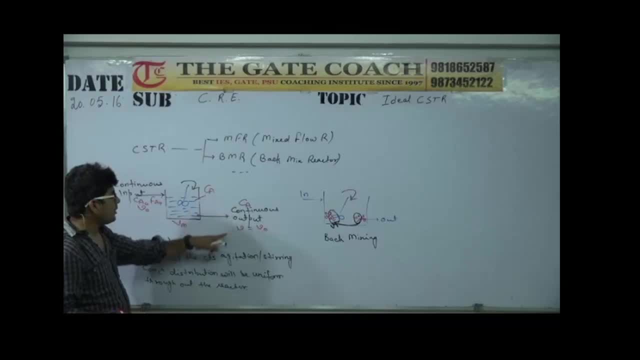 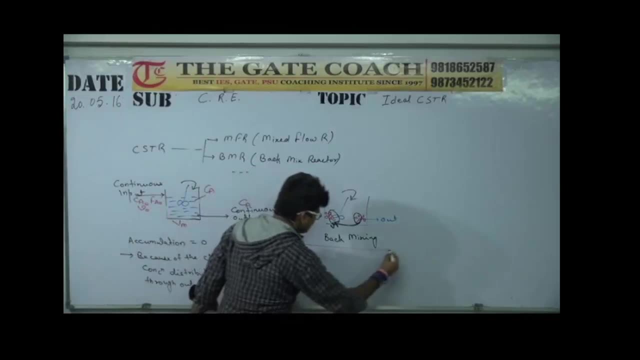 valve will also be same as that of within the reactor. So in this CSTR one important point was this: Concentration distribution was uniform throughout the reactor. And second important point is the concentration at the exit, or you can say if exit is three, 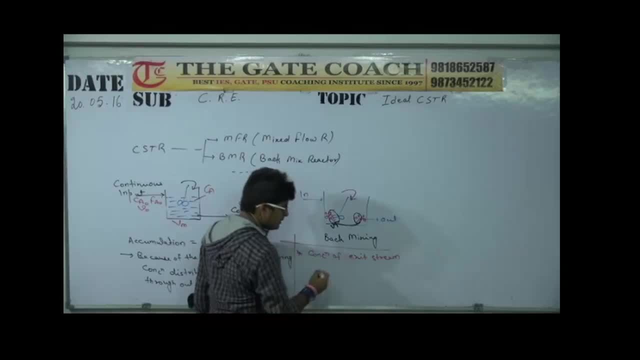 stream concentration. So one more important point is this: concentration of exit stream is same as that of within the reactor. So these are two important points you should know. These are two important characteristics you should know about the ideal CSTR. First, 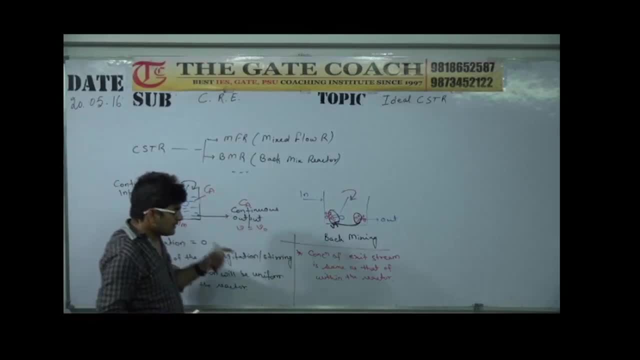 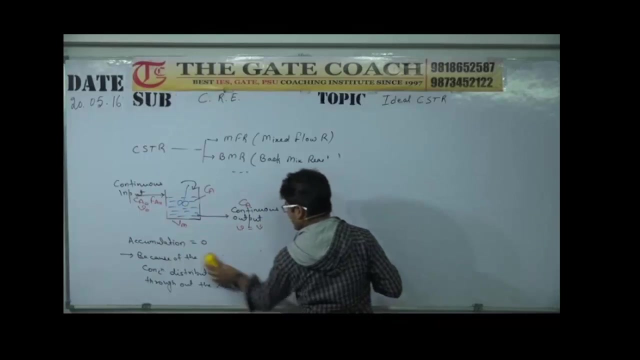 concentration distribution throughout the reactor is uniform and second concentration at the exit will be same as that of within the reactor. So this is something about your CSTR. Now we will talk about design equation of ideal CSTR. Now we will talk about design equation of ideal CSTR. 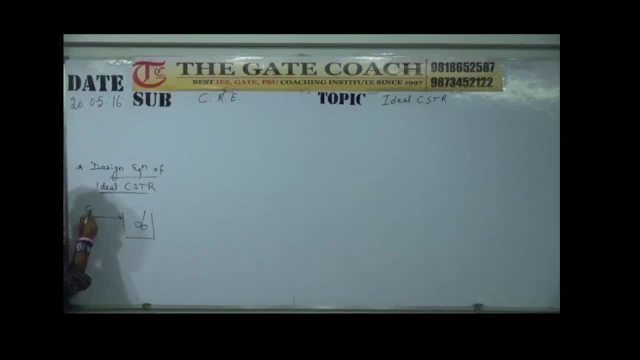 So we have a tank. There is a continuous input. Initial concentration of A is C A. naught. volumetric flow rate V naught. molar flow rate is F A. naught At outlet concentration is C A. volumetric flow rate will be same V naught and molar flow rate is F A Volume. 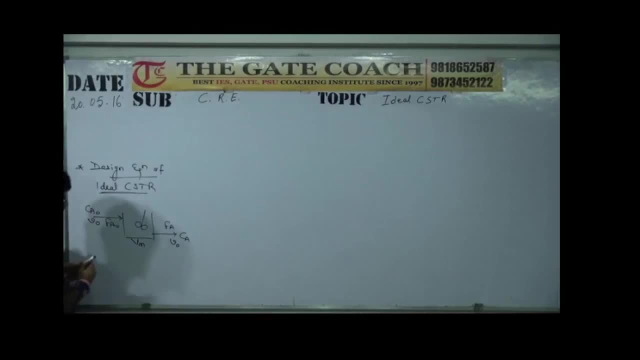 of reactor is V M suppose. So you know that from C A to C A, you know that C A will be equal to C A. So this is the general molar balance equation. What was that? The molar rate of A input is equal to molar flow rate of A input. So this is the general. 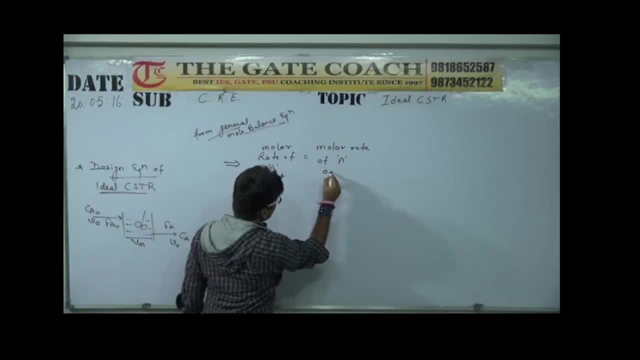 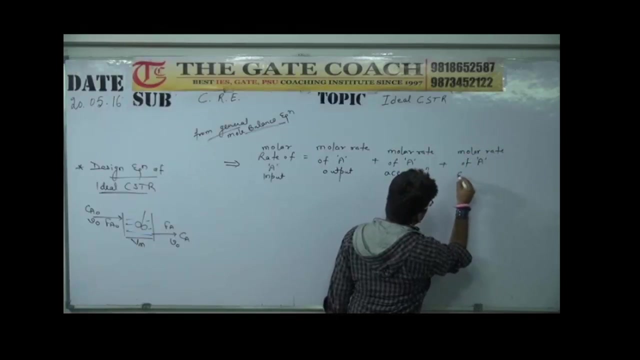 molar rate of A output, plus molar rate of A accumulation, plus molar rate of A disappearance, minus molar rate of A generation. So in this case, because throughout the reactor concentration is uniform, Means at each and every point we have same concentration. So it simply means the average. 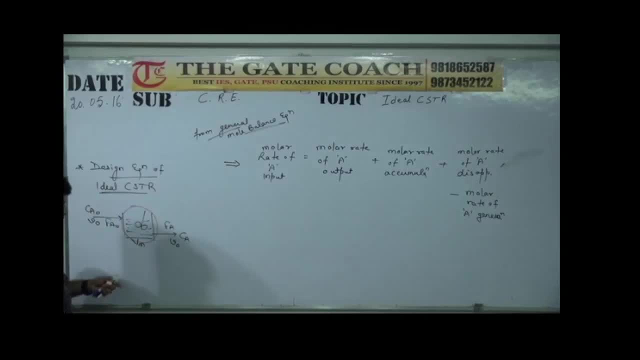 concentration of the reactor will also be same. So we can do overall material balance for this reactor, Because at each and every point concentration is same, So at each and every point component balance will also be same. So we will do overall material balance. 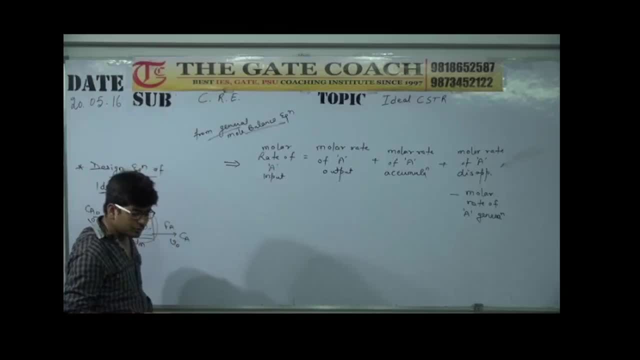 for this reactor. So molar rate of A input – f A naught. Molar rate of A output will be f A. Molar rate of A accumulation – change in moles per unit time – d N A by d t. No, This is a. 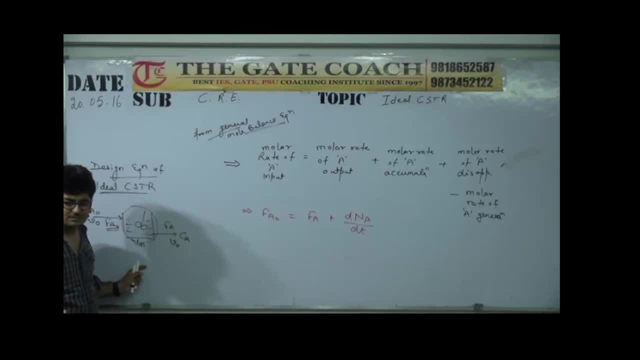 steady state reactor. in this class all the flow reactors operate at a steady state condition. So if this reactor is operating at a steady state condition, so it simply means the accumulation will be zero. Am I right? Yes, I am Plus molar rate of A disappearance, So molar rate of A disappearance. 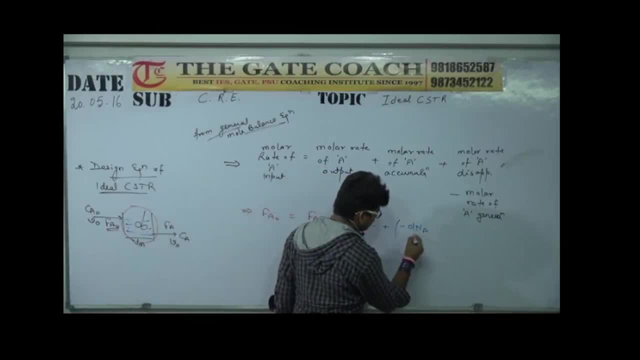 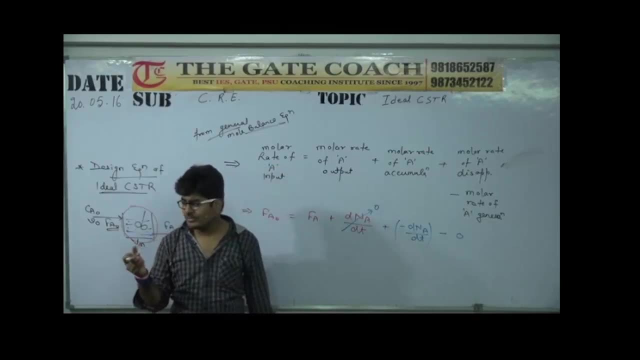 is denoted as minus DNA over DT and molar rate of A generation that will be zero, because we are assuming that A is disappearing in the reaction. The reaction is like this. So tell me one thing: From the rate of reaction for component A we define for unit volume, 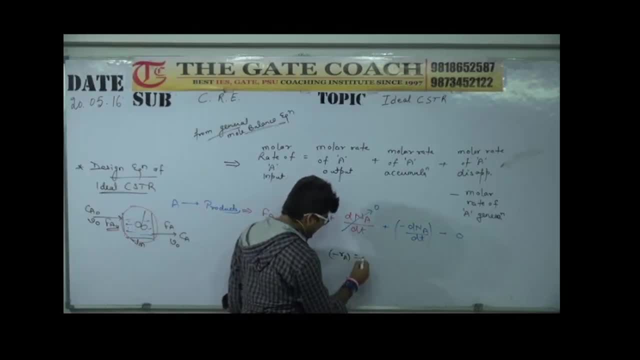 of reaction mixture. We can write minus RA as 1 over V, minus DNA over DT, where DNA over DT is the molar rate of A disappearance. So in this case molar rate of A disappearance will become minus RA into V. Is it clear? Yes, 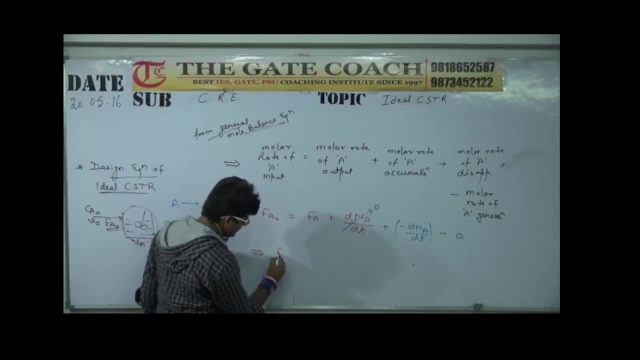 So the final mole balance equation will become FA naught minus FA is equal to minus RA into V. This term. we can write it as RA into V And you know that you can write FA as FA naught 1 minus XA. 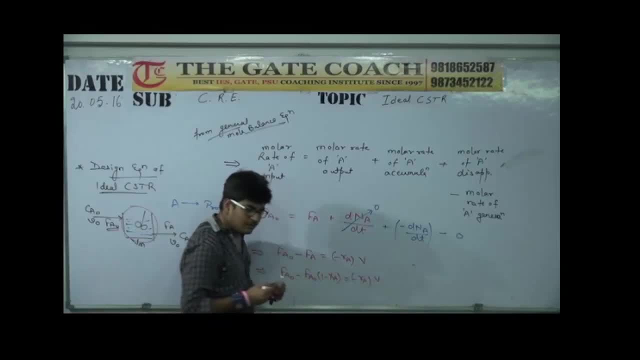 Yes, Yes, See here, V is what, V is a volume of reaction mixture. Say we can write FA like this and V is the volume of reaction mixture. So this equation will become FA naught into XA, into DT, minus A disappearance. 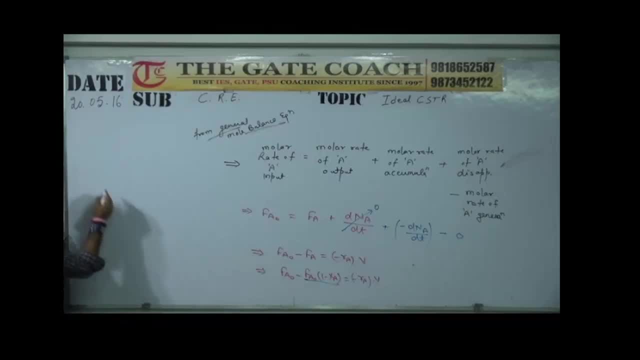 Correct, Correct. Thank you, sir. Thank you, Thank you sir. Thank you, Thank you very much, sir. Thank you also. Thank you, Thank you, Thank you, sir. Thank you very much sir. Thank you, sir. is equal to minus R A into V, or you can write it as V over F A naught is equal to X A over. 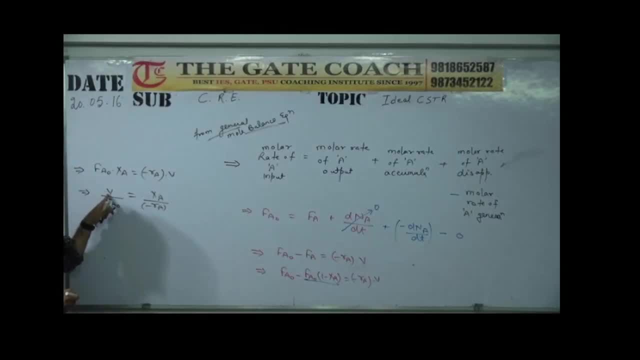 minus R A, Where this V, V is the volume of reaction mixture. and you know that volume of reaction mixture will be same as what? Same as the volume of reactor. See, for example, we have this bottle. This is 1 litre bottle, and how much water does it contain? 1 litre? 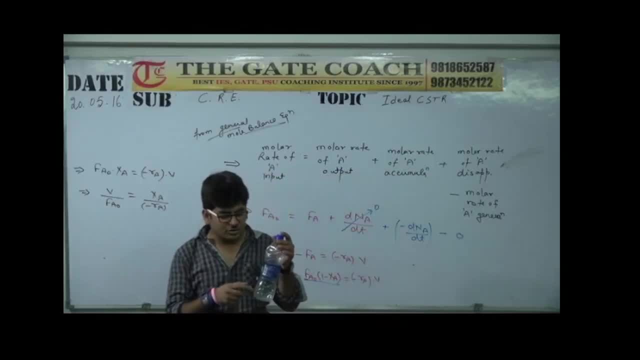 But actually, if you know the actual volume of this bottle, obviously it is more than 1 litre because of some extra volume. we take margin in designing for every equipment. So But if we calculate the volume of this bottle, if we talk about the effective volume, that will be same as the volume of water in this bottle. 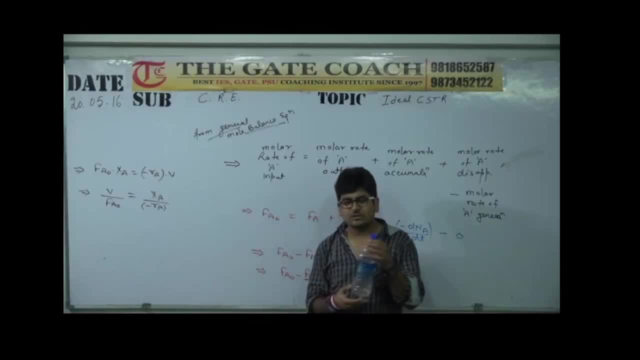 So suppose the volume of this bottle is 1.5L, but we are storing only 1L of water in this bottle. So in calculation, how much volume will you take? You will take effective volume, right, That is 1L. 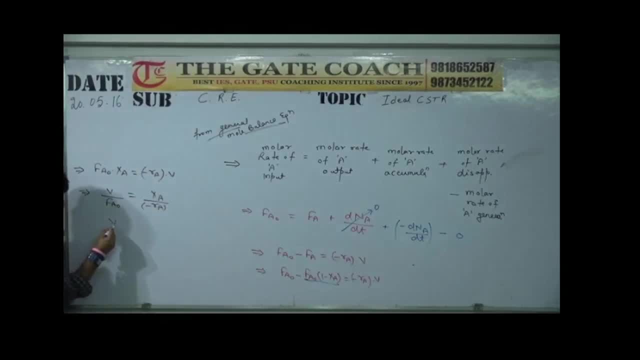 So you can write this: V as volume of reactor And Ra is the rate of reaction. X is the conversion of A achieved in that reactor. Vm is the volume of reactor required. Fa0 is the initial molar force. Fa0 is the flow rate. 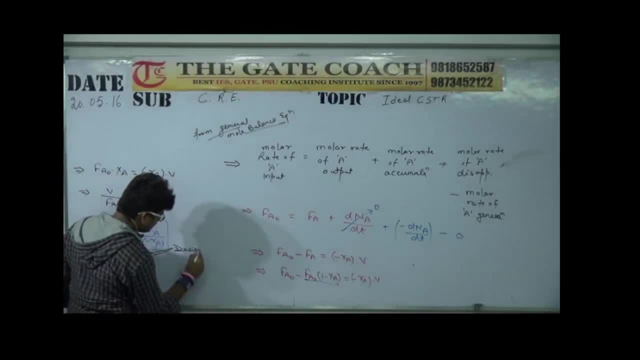 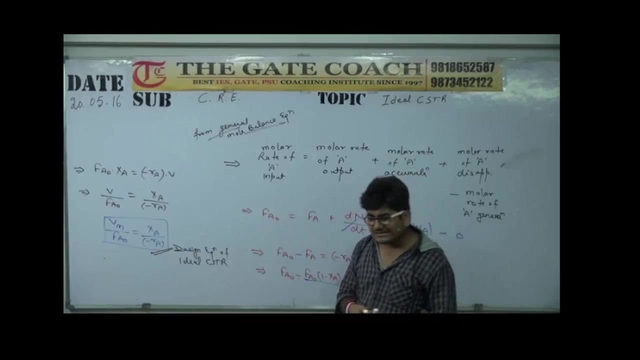 And this equation is design equation of ideal CSTR. So it is clear to all of you. So that's how we design the CSTR. This is the designing of ideal CSTR. We will talk about this in the next class, in next video.